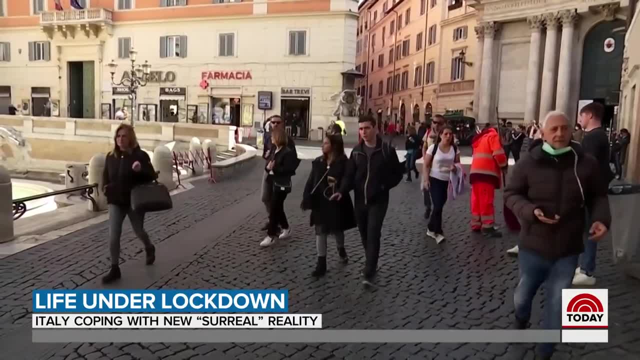 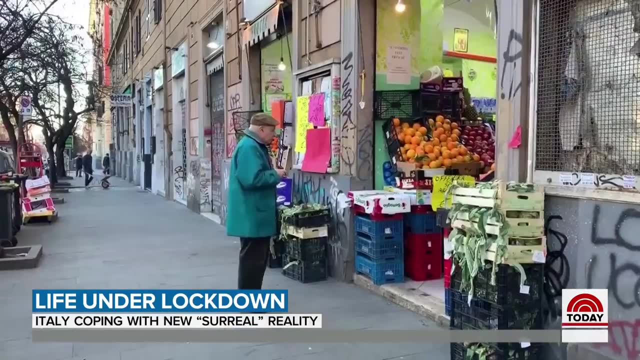 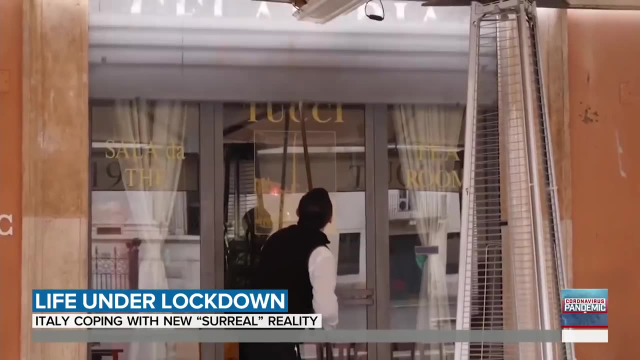 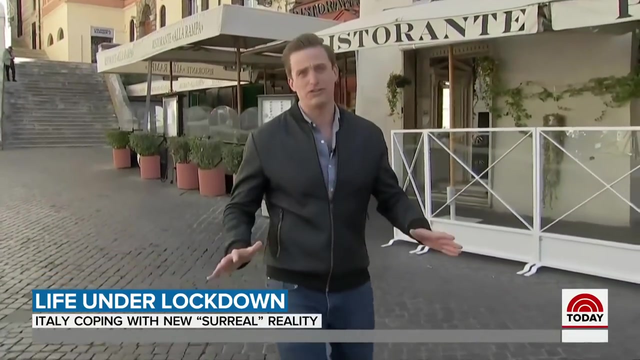 Today in Rome, doing as the Romans do means not doing much at all. Under rules announced late last night across Italy, only food stores and pharmacies will stay open, and so far few reports of stockpiling In the capital. streets are mostly empty. tourist spots are closed and Rome's famous restaurants now shuttered. As of last night, all shops, cafes, restaurants, bars- all forced to close. These restaurants are normally packed with people, but now Italians are going to have to cook for themselves. 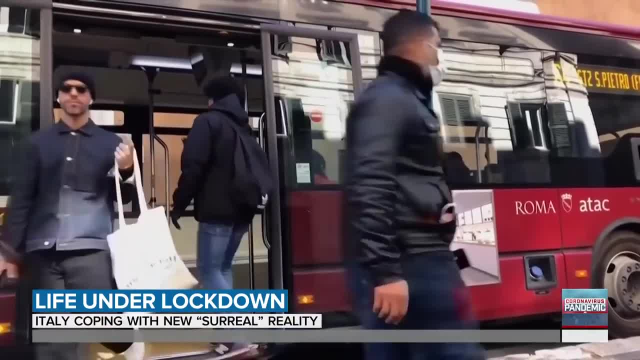 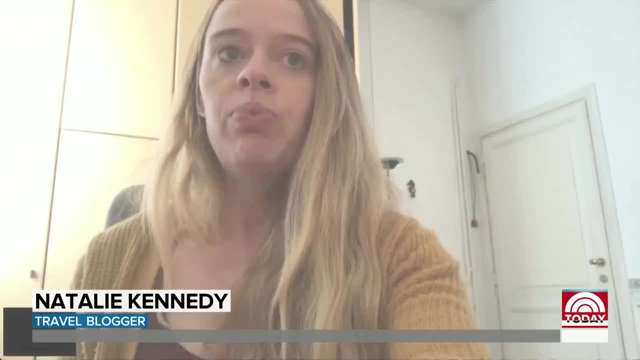 You're allowed to walk around, even go to work if it's necessary, but the government is urging a limit to most activity. The situation started to feel a lot more tense, a lot more real. People are definitely limiting their travel outside of their homes. We're staying home a lot more. 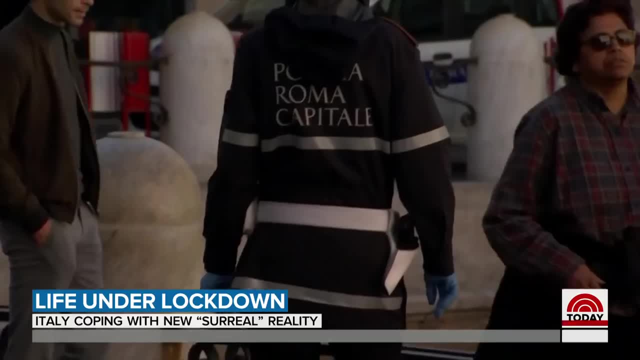 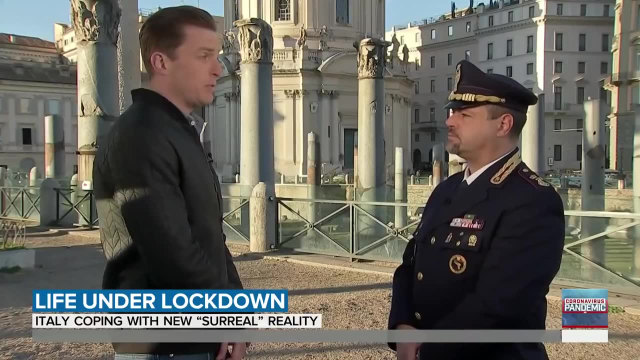 Authorities canceling schools, church services and events, and police telling people to stand at least three feet apart. Violators could face fines, even a few months in jail. Have you imprisoned anyone so far? No, no, no, No, because the people are answering well to this crisis. 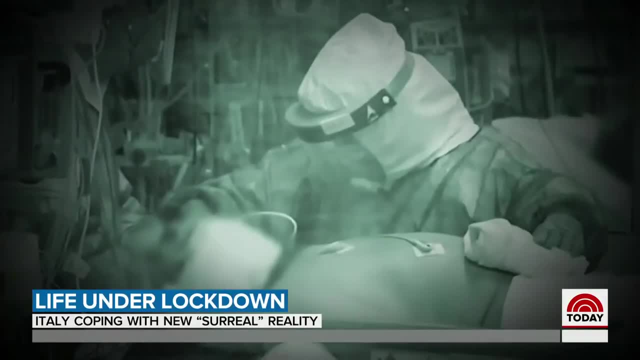 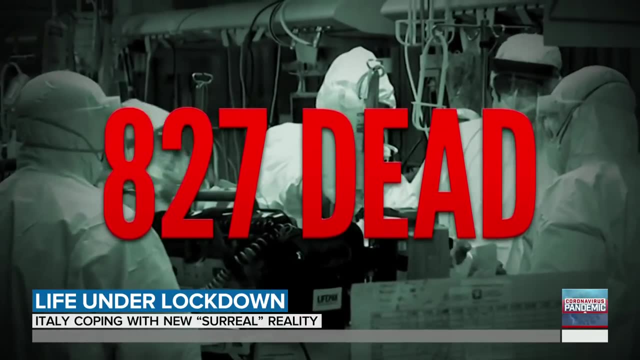 Despite the tough tactics, the virus is still spreading. Italy has nearly 12,500 cases, the second most after China. Yesterday the death toll spiked to 827 dead. but not everyone is worried. You guys aren't supposed to be this close. 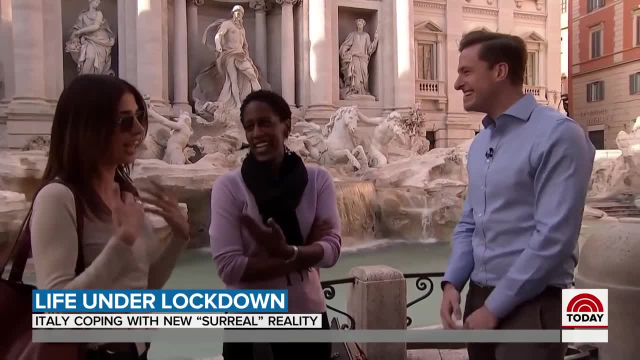 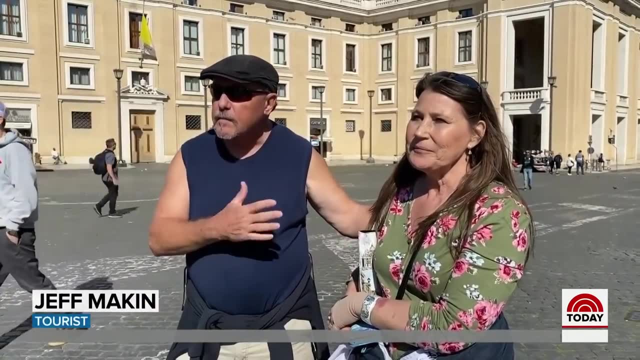 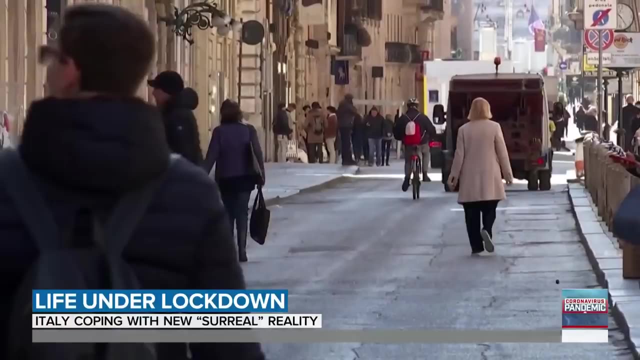 I know, but we're like always this close. We probably got it already. We got it. we'll get it together, While others see it as a challenge to overcome. She has stage four cancer. She's been through chemotherapy, but you have to live and you can't let virus or the flu stop you from living. 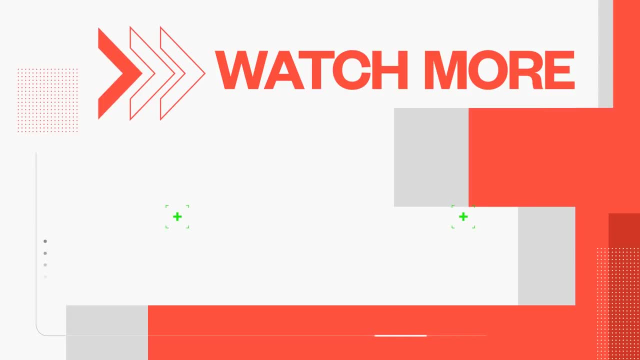 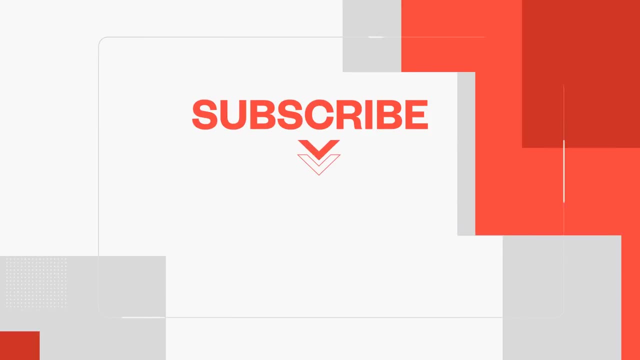